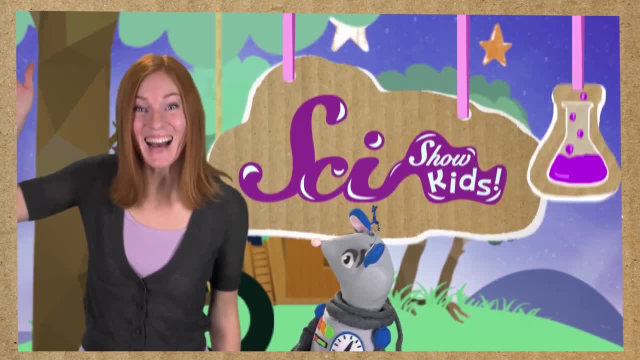 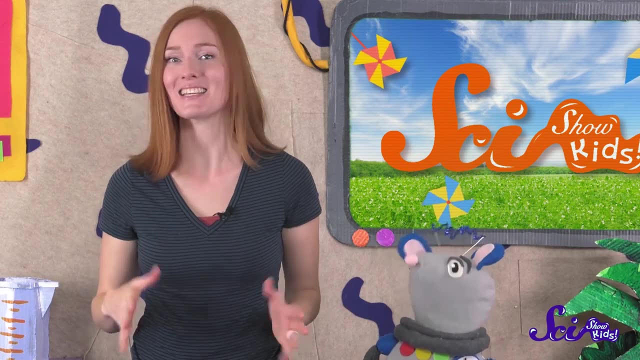 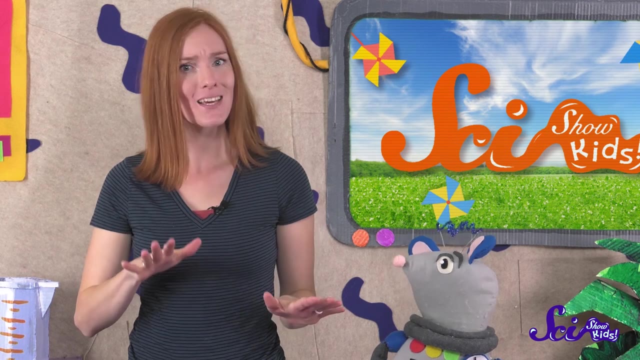 It's a beautiful sunshiny day where we live. My favorite thing about nice days like this is the feeling of the warm sun on my face. But did you know, aside from just feeling nice, the sun's warmth is a kind of energy. 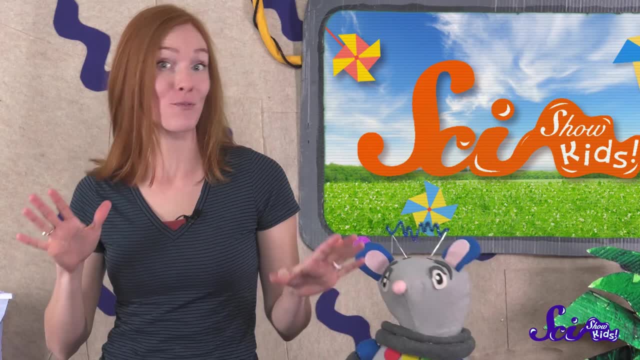 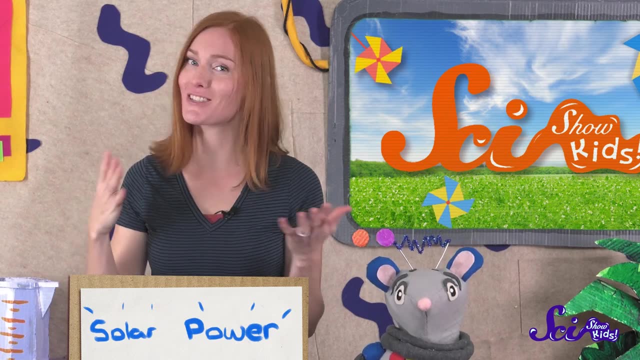 You're right, Squeaks. We use energy from the sun's light and heat for lots of things. When you use the energy from the sun, that's called solar power, because solar is just another word for things that come from the sun. 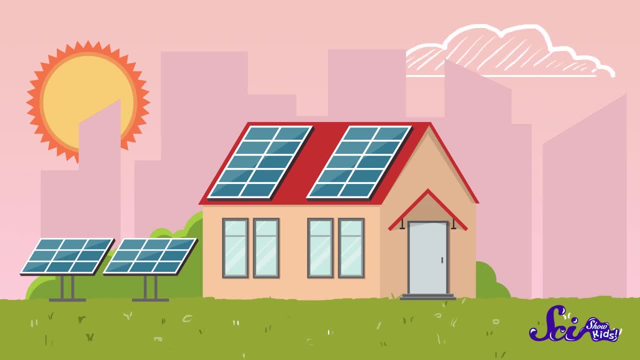 Have you ever seen a bunch of big flat black rectangles on top of a building? Those are solar panels. They take sunlight and turn it into electricity. Some people also collect the heat from the sun to warm their homes or heat their water. 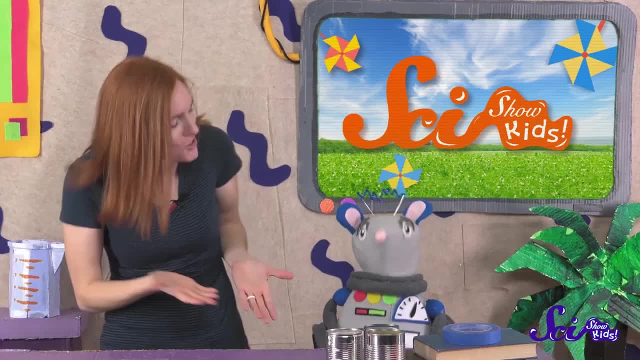 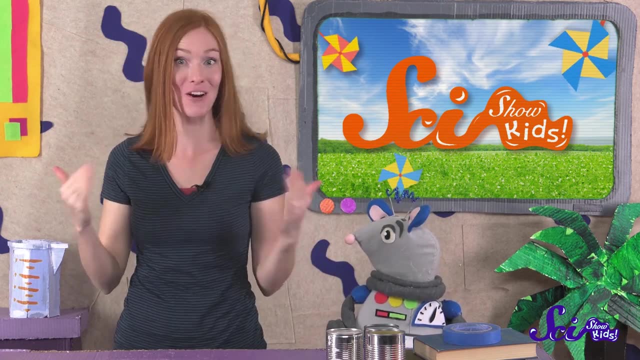 I even built Squeaks to run on solar power. You know Squeaks. this warm, sunny day got me thinking about a cool project that we could do together to use the sun's energy ourselves. Do you want to try it out? 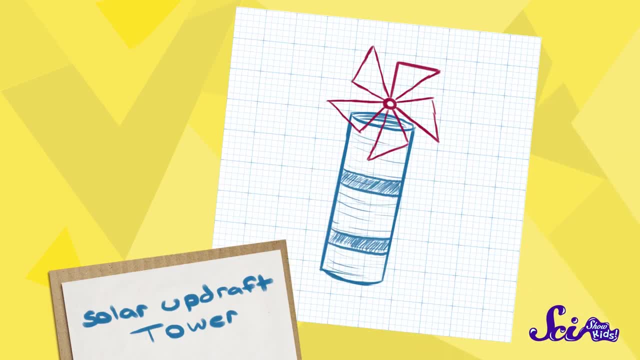 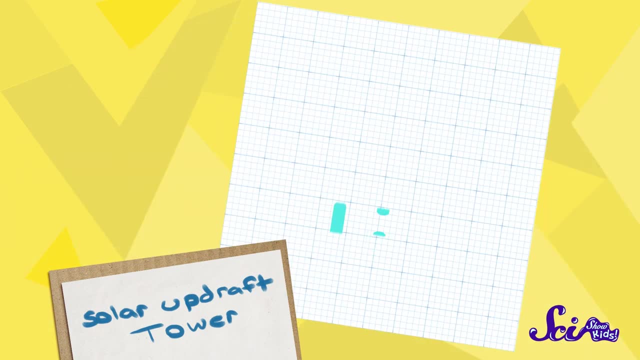 Okay, let's do it. We're going to build something called a solar updraft tower. Since it has the word solar in it, you already know that it has something to do with the sun. Updraft just means a kind of wind where the air moves up. 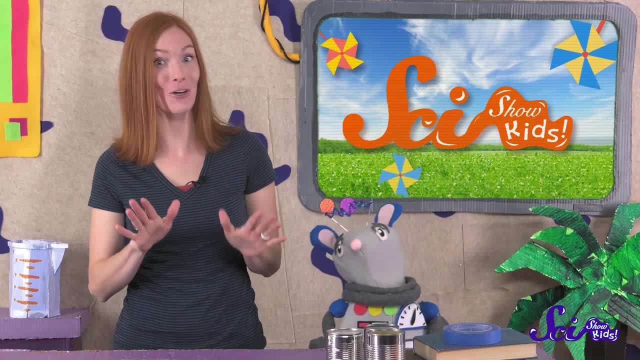 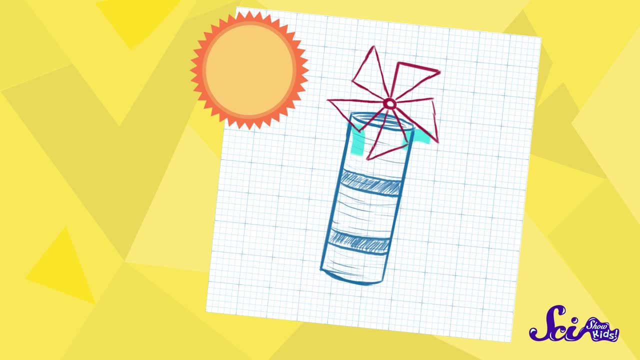 And you know what a tower is. So can you guess what our solar updraft tower will do? It'll take sunlight and use that to make air move upward through a tower and spin a paper pinwheel. You can try this project at home too. 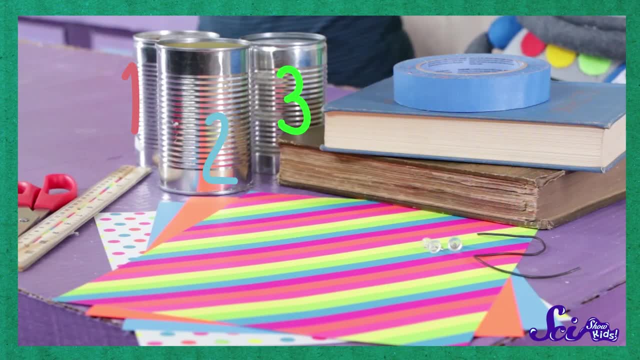 First, you'll need three clean tin cans with the tops and bottoms cut off. You'll also need some tape, a piece of wire like a paperclip, some thumbtacks and two books that are about the same size. They need to be pretty big books. 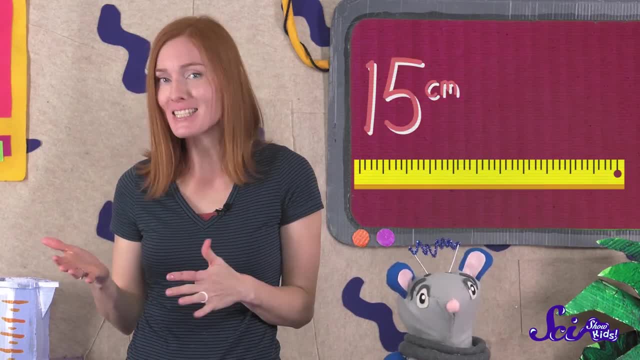 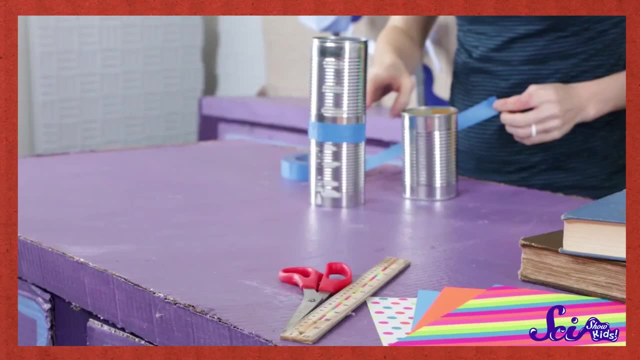 Then ask a grown-up to cut a piece of paper into a square- 15 centimeters, or about 6 inches on each side. And, most importantly, you need a sunny day. Now we're going to build the tower First, stack up the cans and tape them together really well. 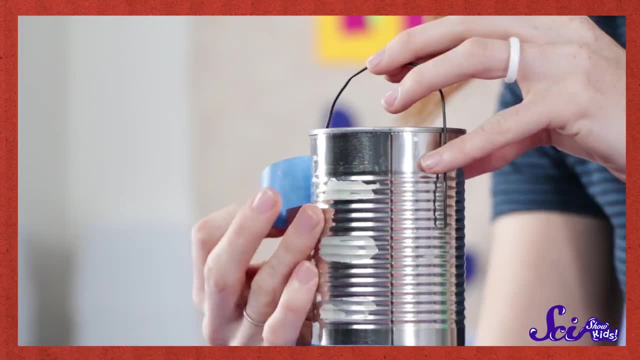 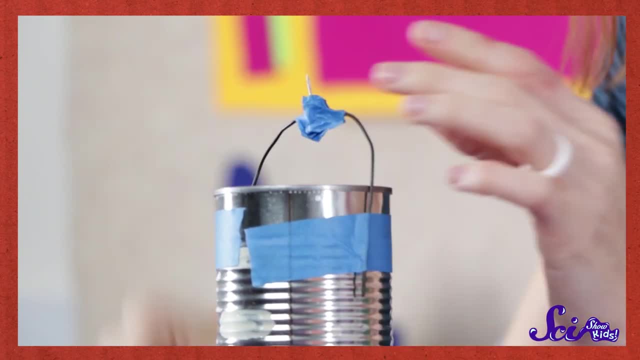 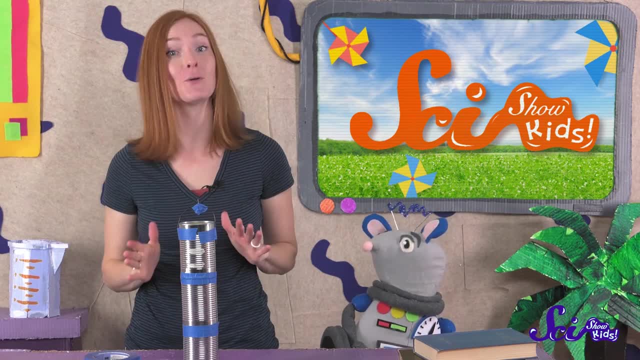 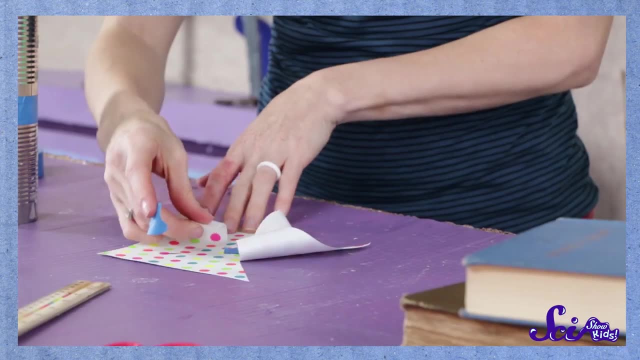 Now we'll fold the pinwheel. Grab your square paper and have your grown-up help you cut diagonally from the corners. Don't cut all the way through the paper, though — stop cutting about this far from the middle. Once all of the corners are cut, fold them like this and tape them together in the 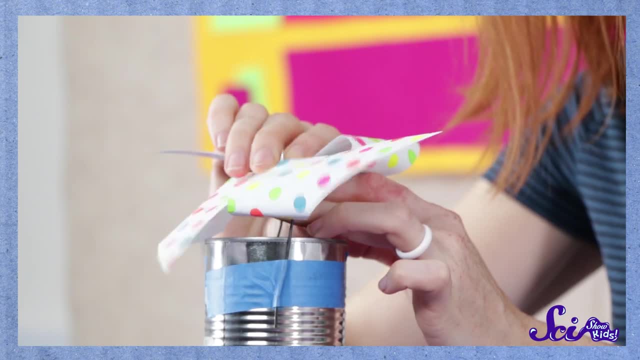 center. Then get your grown-up to stick the pinwheel onto the pointy end of the tack And our tower is ready. All we have to do now is put the can tower on top of the books, so there's a gap at. 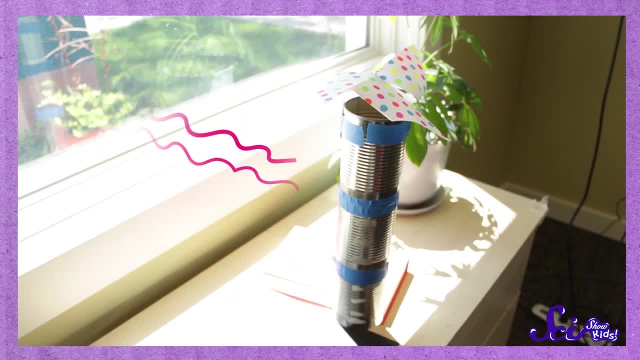 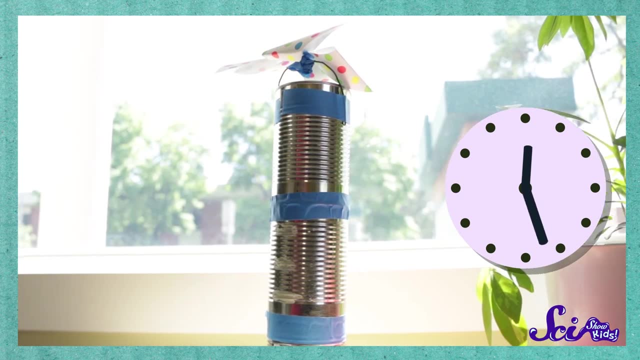 the bottom and set the whole thing near a window where there's direct sunlight coming through direct sunlight, so the sun is shining straight through the window. It might take a while, depending on how warm and sunny it is where you are, so be patient. 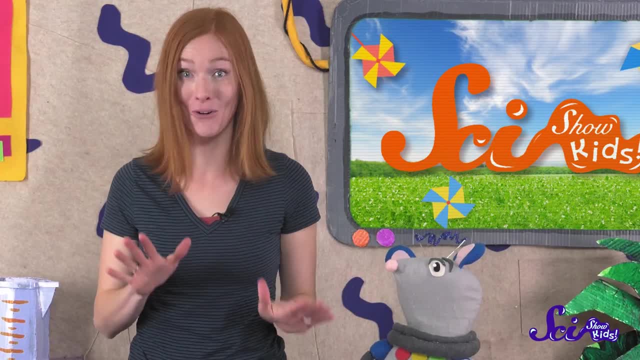 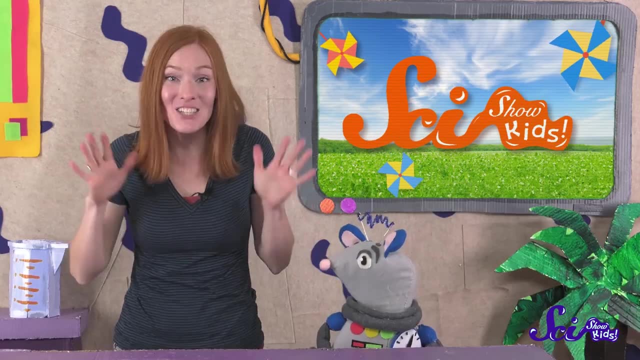 and check on your tower every now and then. After a while, something really cool will happen. Whoa, The pinwheel is spinning. It's not magic Squeaks, It's science. When the sun shines on the cans, they get hot. 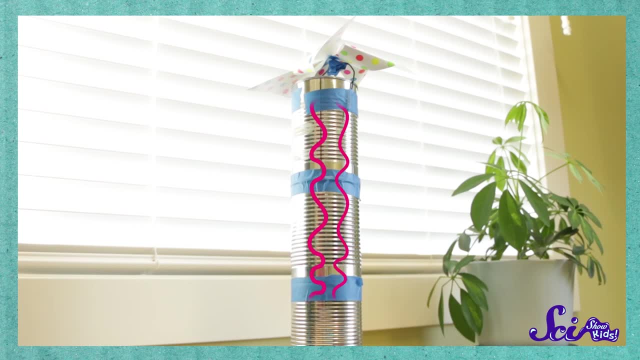 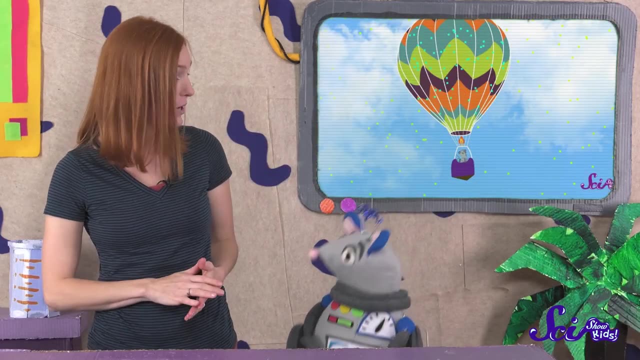 Some of that heat travels through the metal to the inside of the cans, so there's hot air inside the tower And hot air rises Squeaks. do you remember when we learned about how hot air balloons work? Well, this is the same kind of idea. 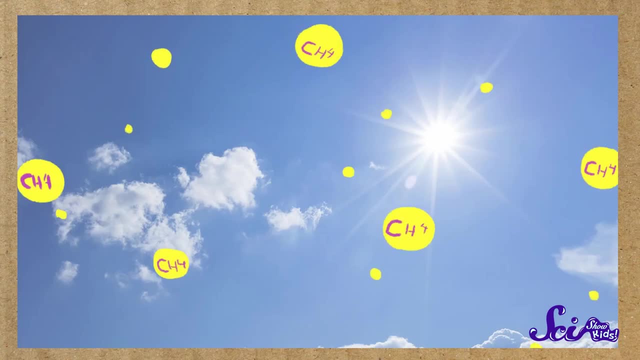 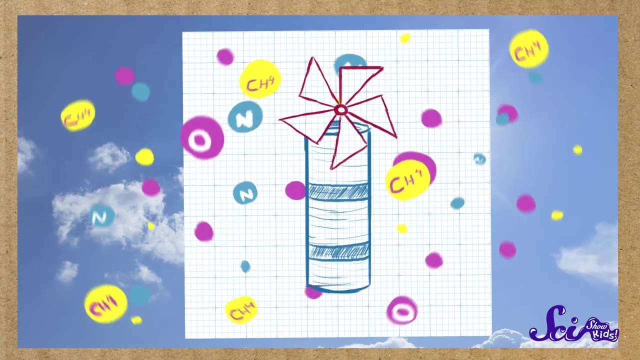 Air might seem like it's made of nothing, but it's actually made of lots of little tiny particles, way too small to see. When sunlight heats up the air inside our tower, the heat makes those tiny little particles start to bounce around faster and faster and spread out. 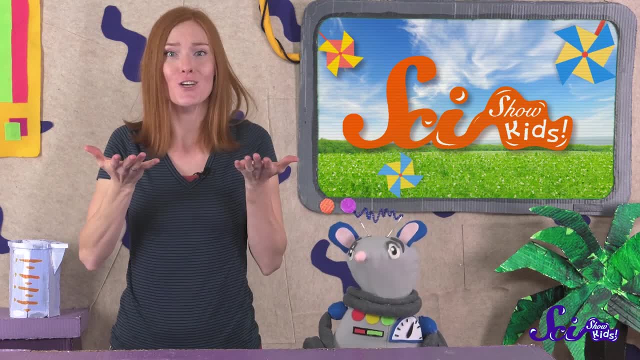 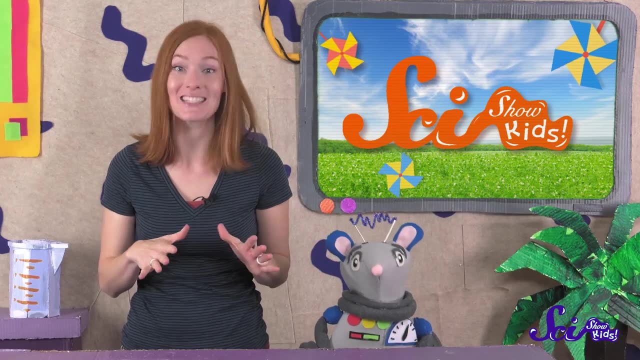 Warmer air that's more spread out like that will move upwards, so it's on top of the cooler air that's less spread out. It's a lot like how a plastic spoon will float on water In our tower. that means that when the sun warms up, the air inside the cans the warmer. 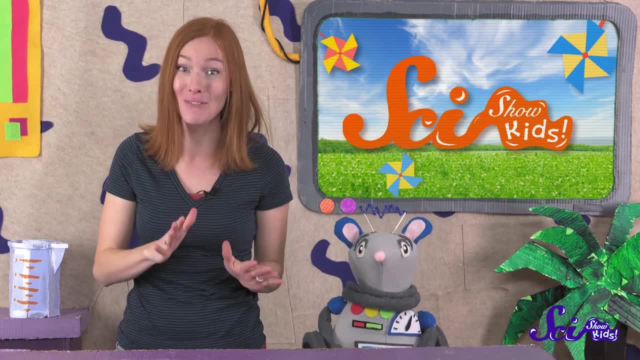 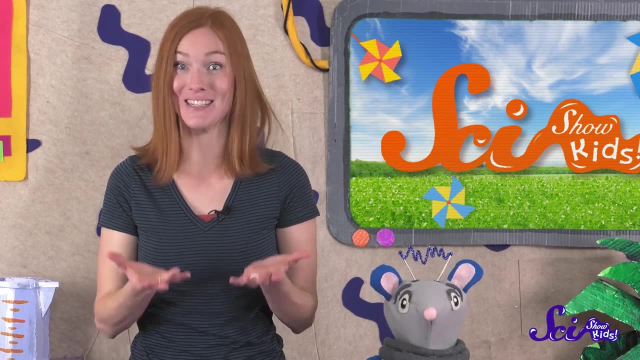 air will move upward through the tower and make the paper pinwheel spin as it passes by. Then cooler air comes in through the gap at the bottom of the tower, gets heated up and rises, so there's a constant flow of warm air that keeps the wheels spinning. 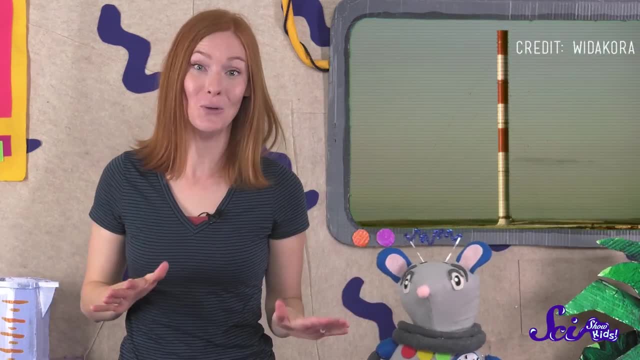 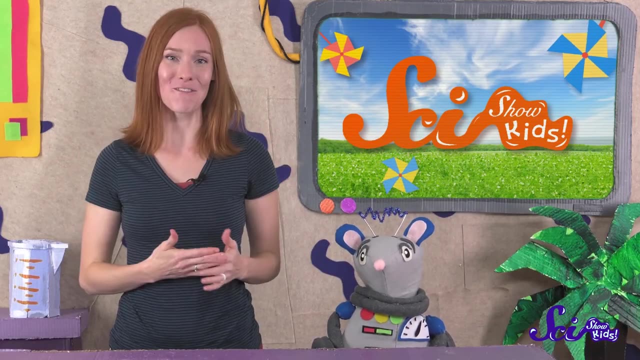 We've made a solar updraft tower. There are some places in the world where they actually use giant solar updraft towers to generate electricity. So the next time you feel the warm sun on your face, remember that it's more than just a nice feeling. 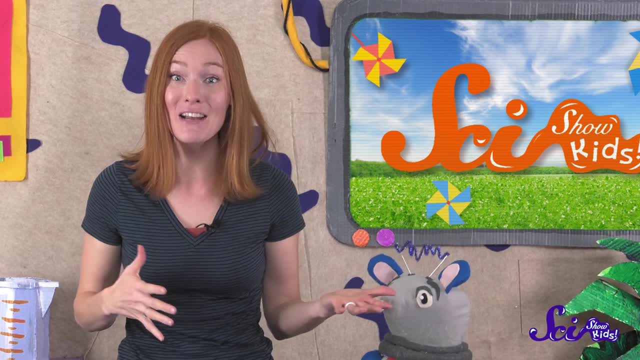 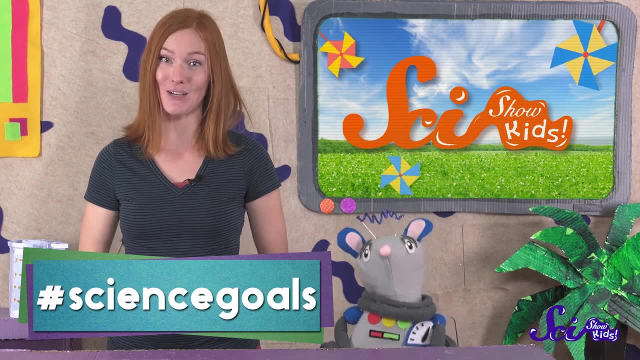 Sunlight is a powerful and useful source of energy. It's the same energy Squeaks uses to get around. Thanks for joining us on SciShow Kids and thanks to Google Making Science for helping us with this episode. Did you make a solar updraft tower of your own?